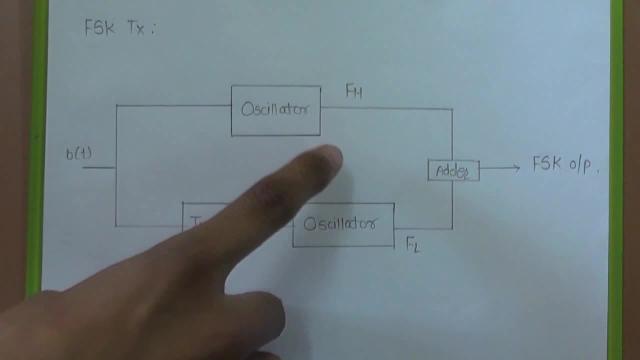 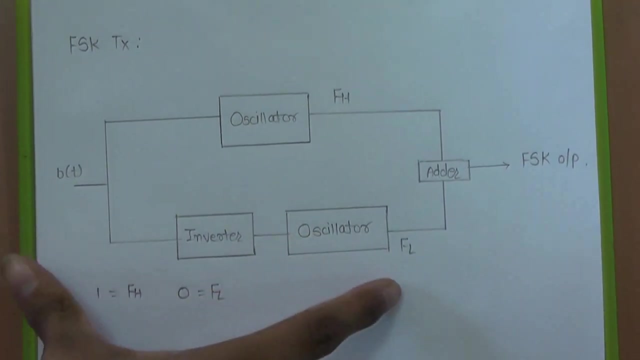 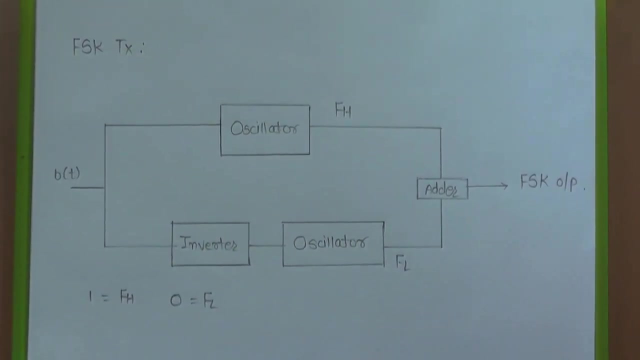 be generating a higher frequency FH, While if 0 is transmitted, it will be inverted to 1 by the inverter Oscillator. 2 will be producing a lower frequency FL. Both the frequencies will be added and FSK output is generated, Where first bit 1 will be corresponding to. 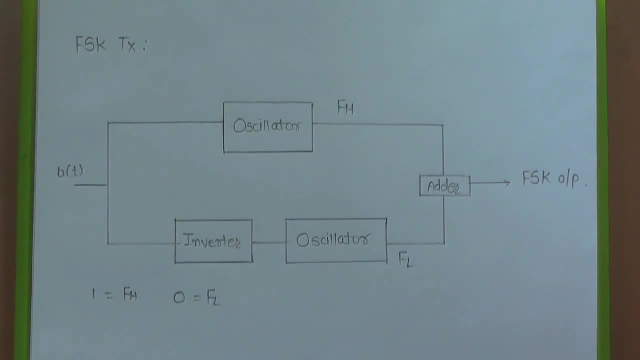 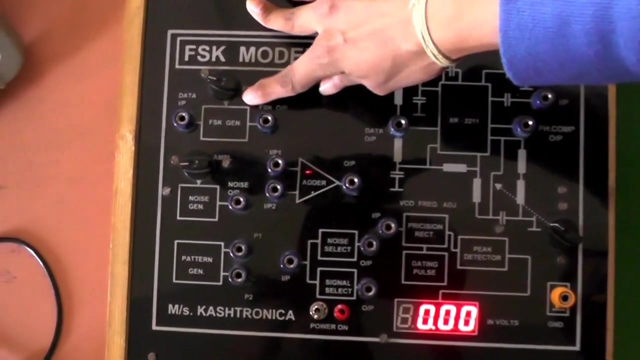 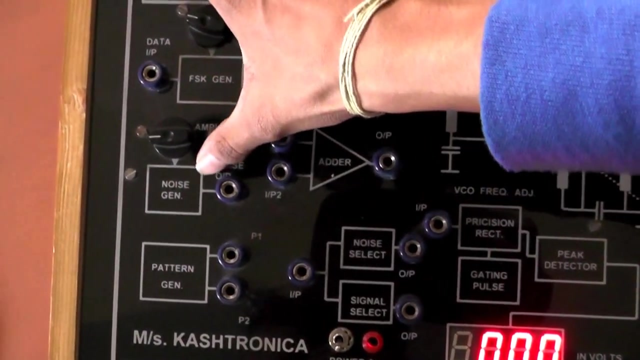 higher frequency and 0 bit will be corresponding to lower frequency. Here we have the FSK modem. It consists of the FSK generator to generate the FSK signal, a pattern generator to give the input stream of bits, A noise generator to generate the noise at the input side. adder to add noise and FSK. 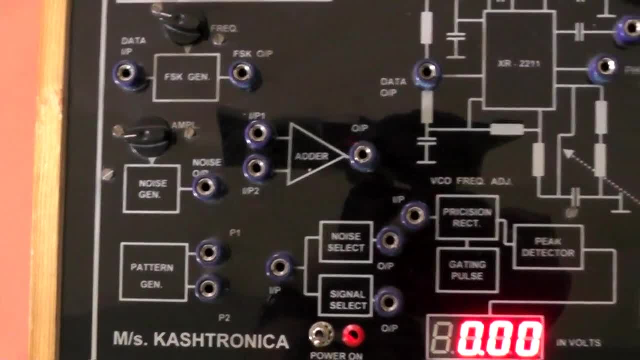 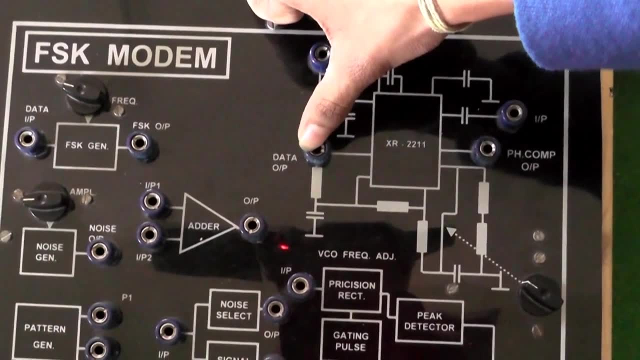 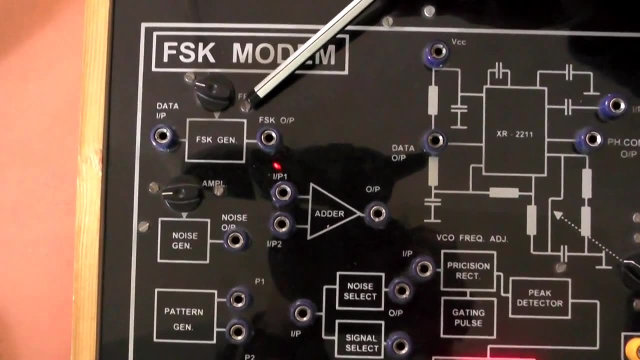 signal. for getting the distorted FSK signal Here it consists of the FSK receiver, which will give the input data stream back. The first step. it will be consisting of measuring the carrier frequency First of all at the transmitter side, it will give the input data. 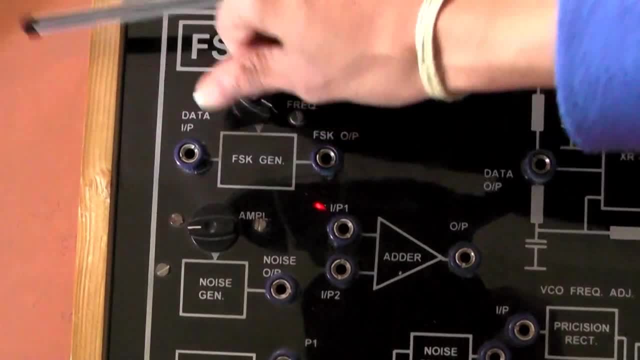 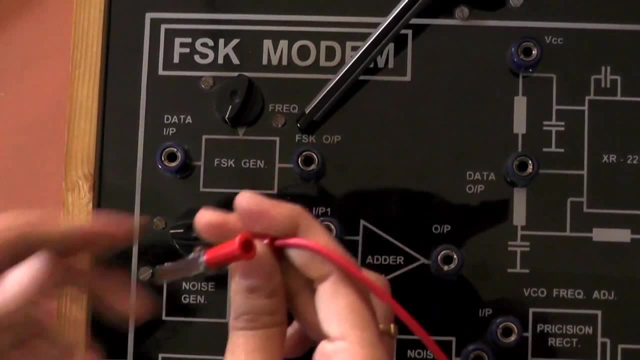 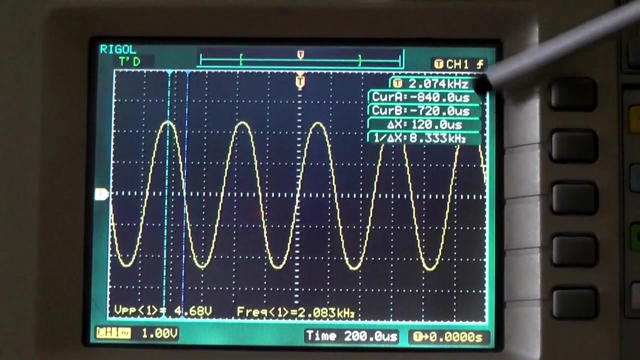 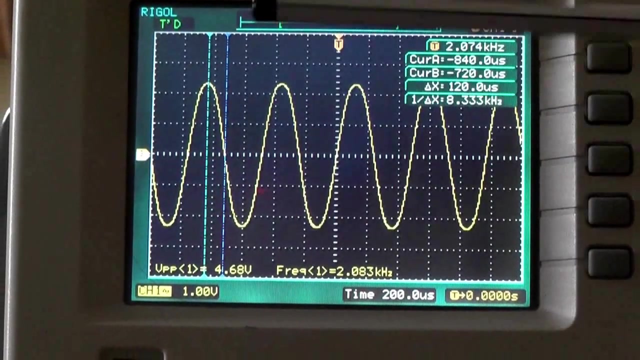 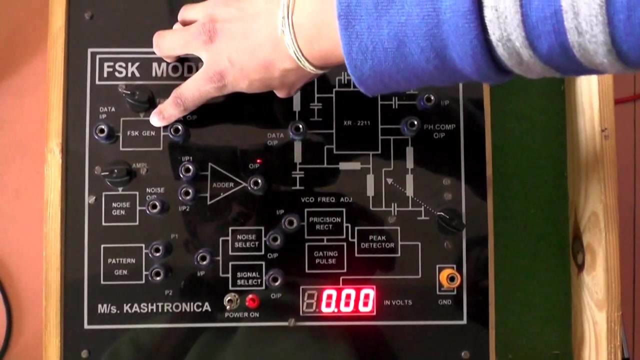 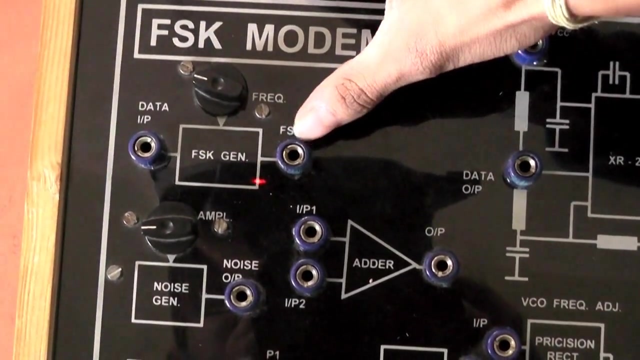 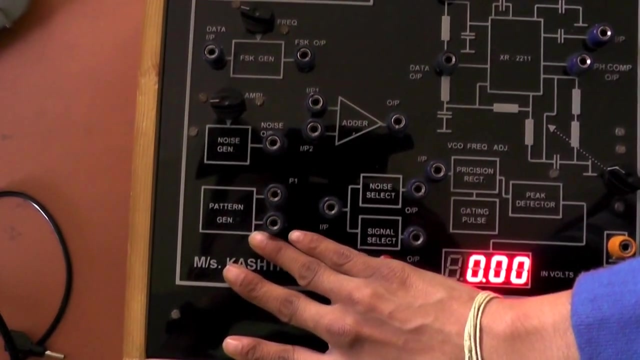 stream back At the transmitter side it will be talking to the food signal. First step in the transmission is the carrier signal. Of course a load or dispg FSK generator is used to generate the FSK signal Without giving any input. the output is measured to get the carrier frequency And your pattern generator. we check for the pattern for generating the FSK signal. 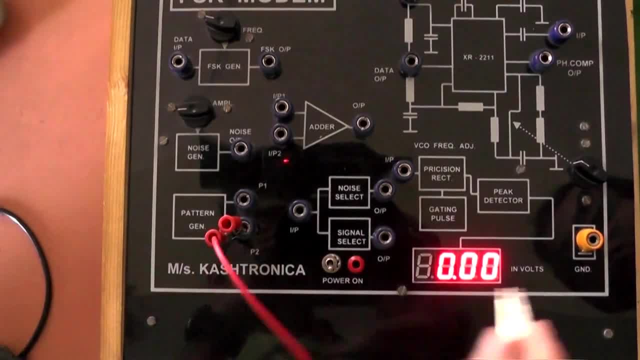 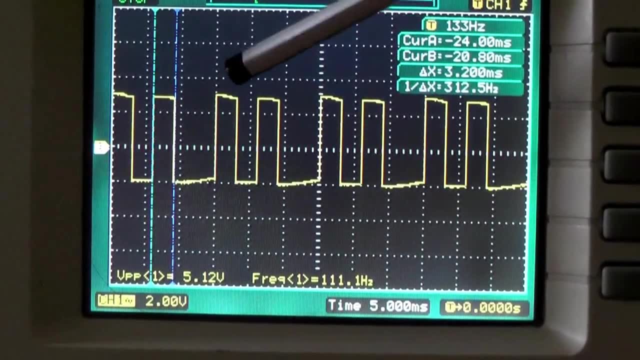 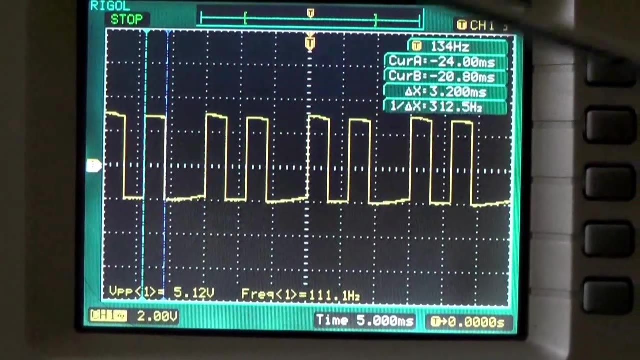 Here on the DSO we can see the pattern generated. Here we can see the pattern generated is 10100.. We will check the bit duration, TB, using the cursor. Here we get the bit duration as 3.2 ms, that is approximately 3 ms. 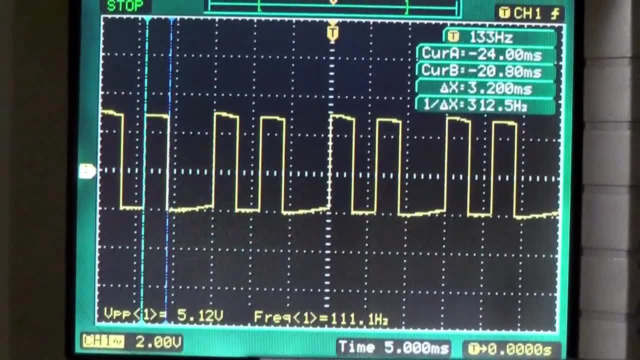 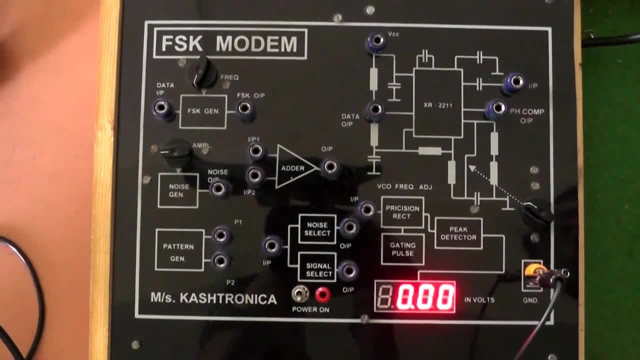 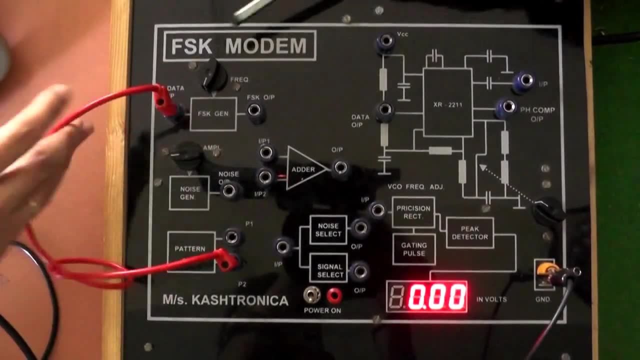 The V peak to peak is 5.12 volt And frequency of the entire signal is 100 hertz. Step 3, we will give the pattern generator output to the data input of FSK generator and check the FSK output And observe it on DSO. 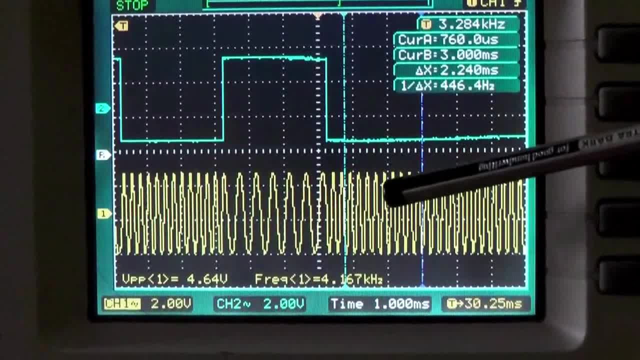 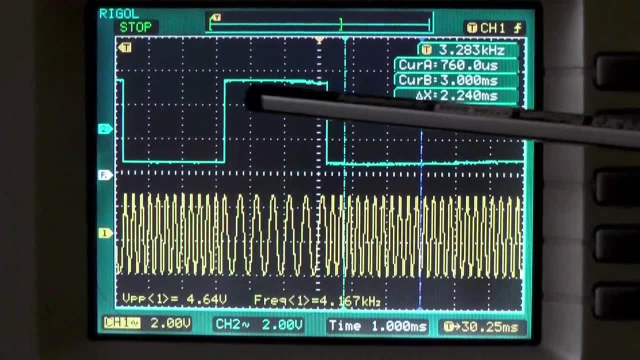 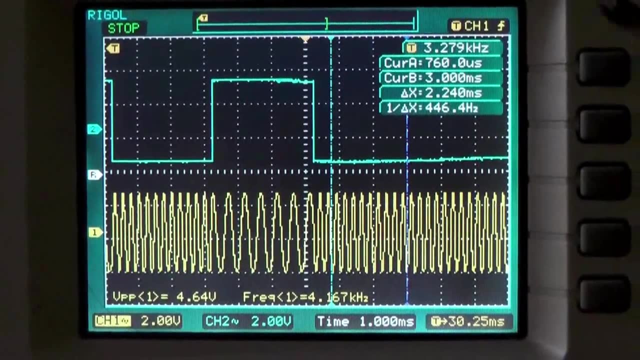 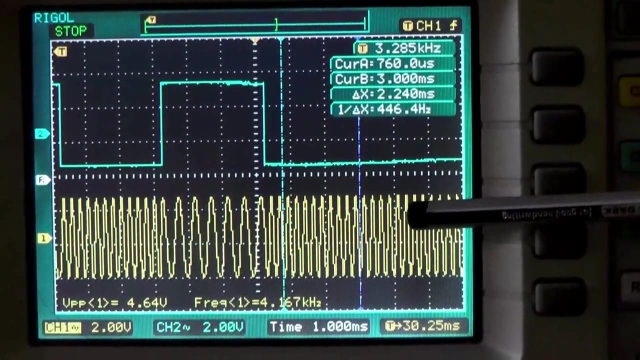 Here on the screen we have the bit pattern and the FSK generated signal. So here we can see exactly where the frequency is, From bit 1 to bit 0, we have high frequency and lower frequency. Here the input circuitry is such that for bit 1, a lower frequency is transmitted, while for bit 0, a higher frequency is transmitted. 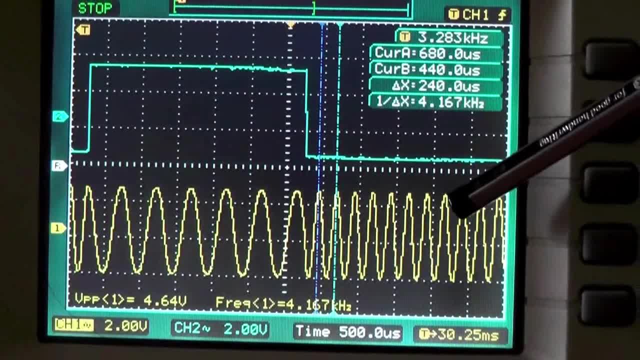 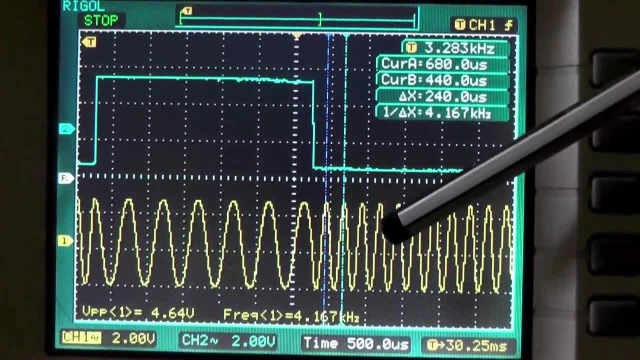 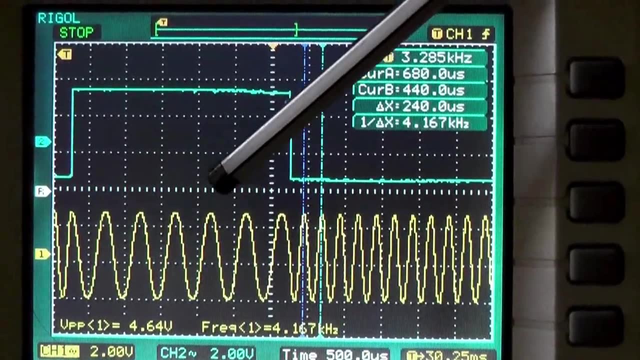 For the FSK signal measure higher frequency FH and lower frequency FL. Here we have the cursor set for the higher frequency. We get it approximately 4 kilohertz. Similarly, we can measure the frequency for FL, and it will be approximately 2 kilohertz. 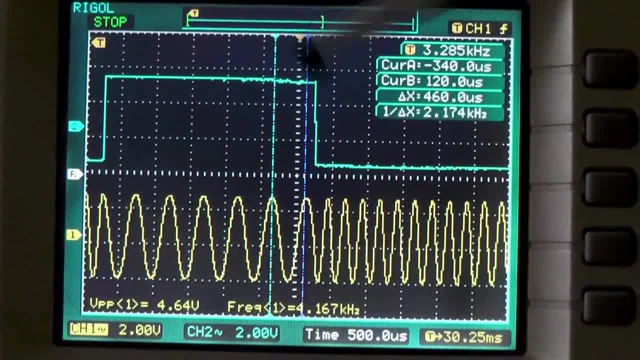 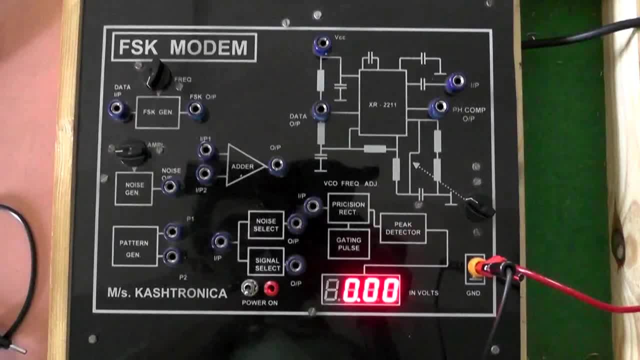 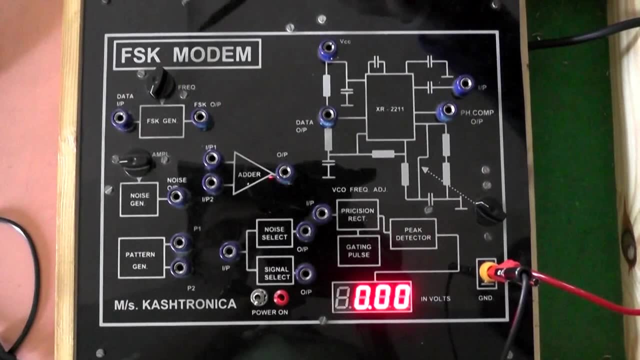 We have the cursor set for measuring FL, And here we can see that FL is equal to 2 kilohertz. In this experiment we have to compare the signal to noise ratio at the input and at the output. So at the input. 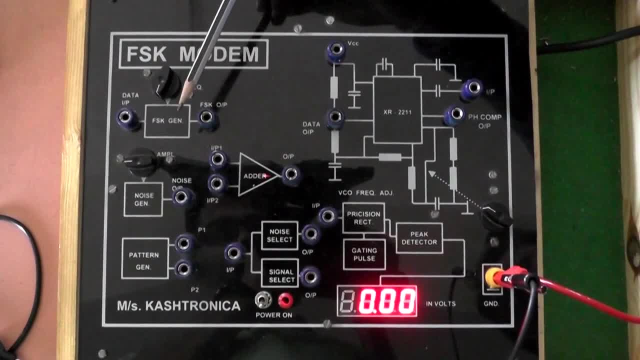 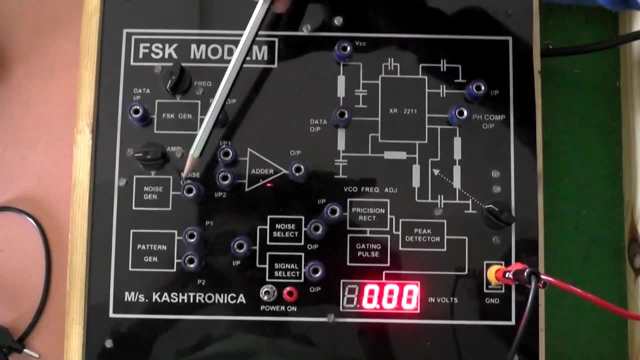 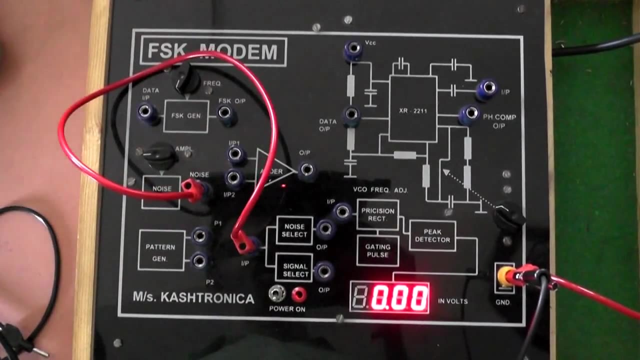 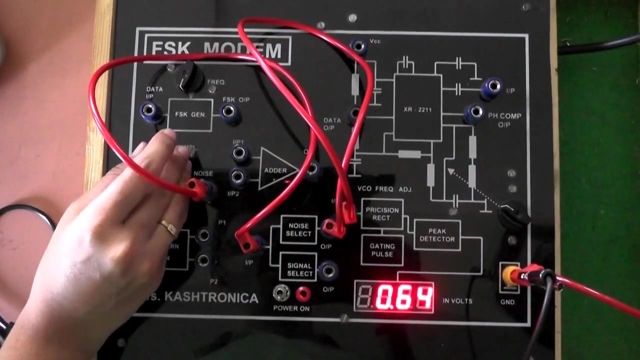 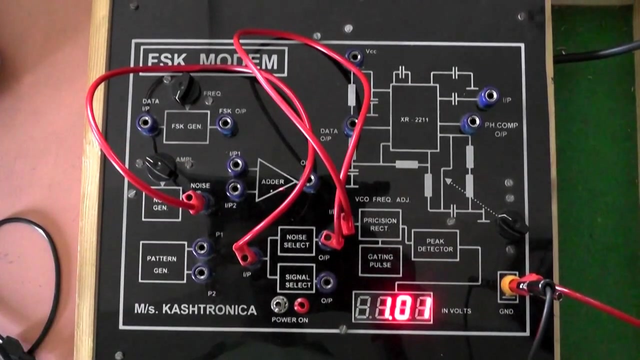 We will add the noise of 1 volt as a reference. 1 volt as a reference. to generate the noise of 1 volt, We will first set the noise as 1 volt. After setting the noise at 1 volt, we will give the noise to adder.